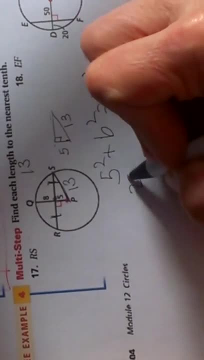 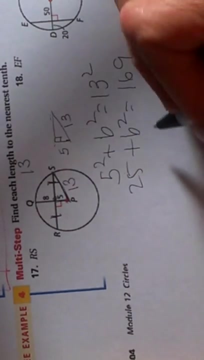 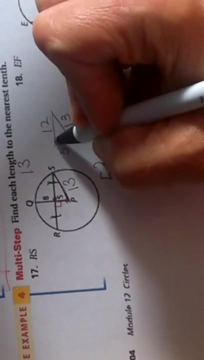 Pythagorean Theorem. I don't know if you recognize this, but this is one of the triples that Ms Sphere was talking about. So 25 plus B squared is 169.. So B squared is 144.. So guess what B is? B is 12.. So that's 12.. So that segment is 12, which. 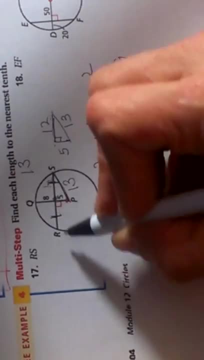 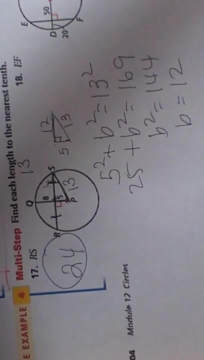 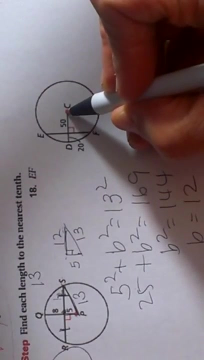 means from the center to S is also 12, which means R to S has to be 24.. That's how you do it. That's how you do all of these. So let's look at 18.. You have from C to here. 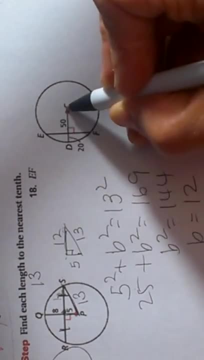 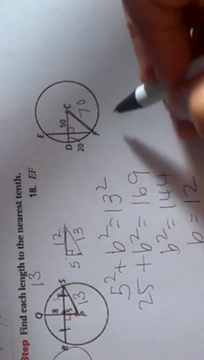 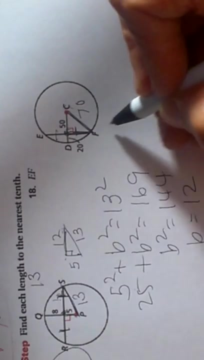 is 50.. From here to D is 20.. So that means CD. the radius is 70. So draw your radius here, and that is 70.. Use the Pythagorean Theorem. Let's find this segment from this point here down. This time I will treat it as A A squared. 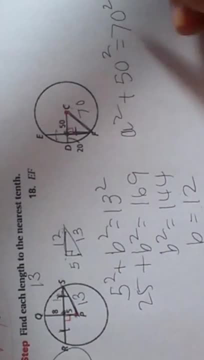 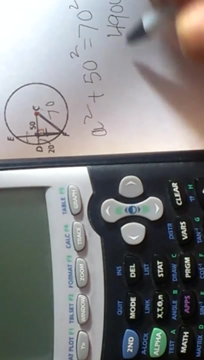 plus 50 squared equals 70 squared. Pythagorean Theorem again. So let's see, 70 squared is 4900.. 5 squared is 2500. plus A squared, Let's see that is going to give us 2400.. So that's. 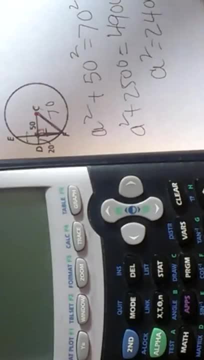 400. and that's not a perfect square, is it? No? so let's just break it down. If we divide it by 2, that's 2 times 1200.. Actually, let's do it like this, Let's do 60 times 40 and. 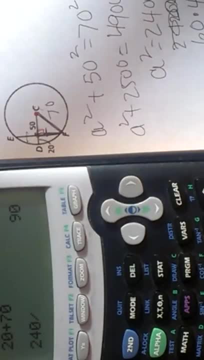 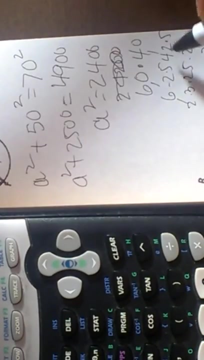 do that as 6 times 2 times 5.. That's 4 times 2 times 5.. That's 2 times times 2 times 5 times 2 times 2 times 2 times 5.. So let's start taking pairs out. Let's. 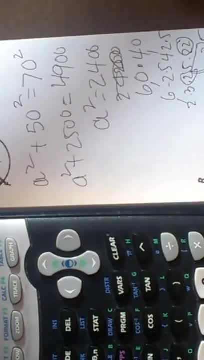 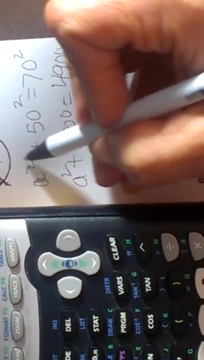 see a pair of 2's, another pair of 2's and then a pair of 5's. So that's 5 times 2 is 10 times 2 is 20.. So 20 root 6.. There we go. Ok, 20 root 6, that is the length from here.